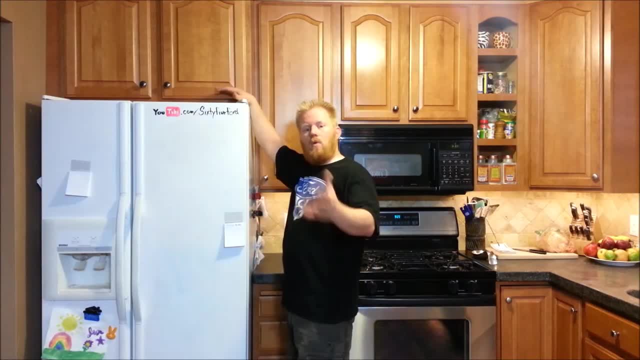 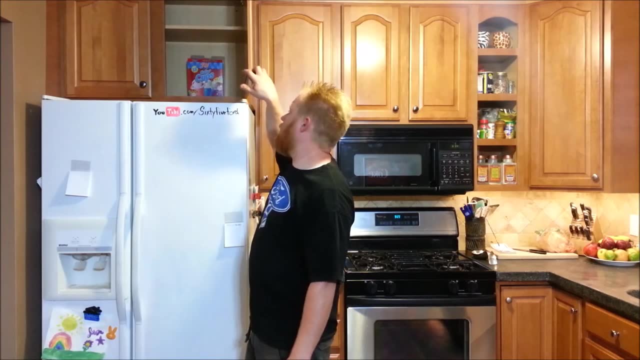 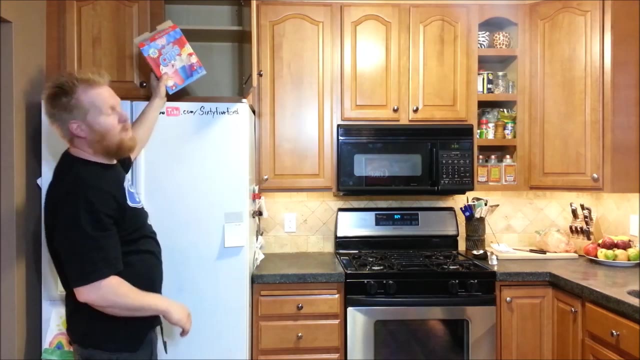 But everybody that has a cabinet above the fridge knows how horrible it is to actually use it. get anything in and out of it. This one, because it's pulled out, I can't reach it, I can't open it, But the stuff at the back got my ice cream cone right here. you know it becomes extremely hard to reach and utilize. 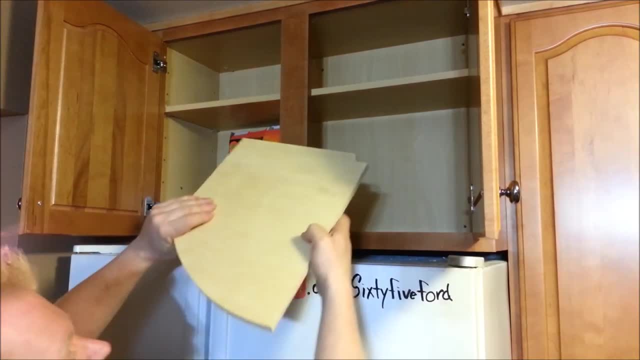 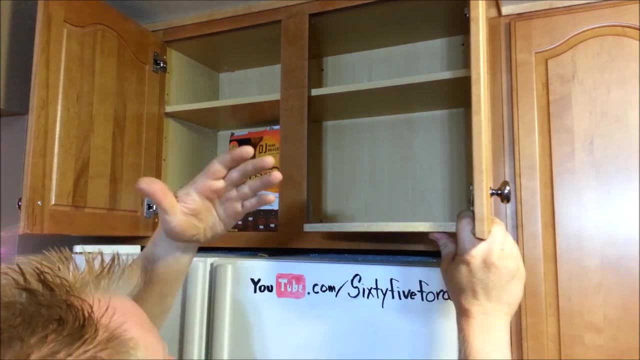 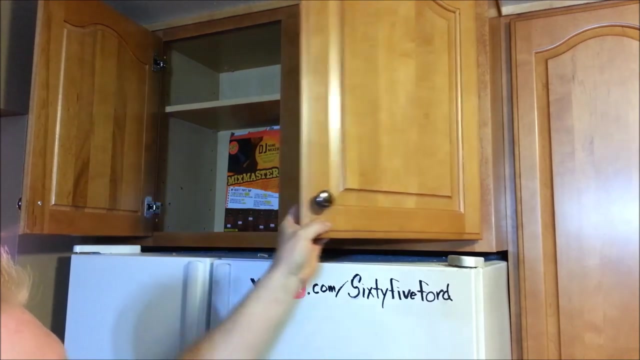 So we're going to fix that. So, essentially, what we're going to do is make a shelf. A shelf that comes out when you open the door and actually retracts when you shut the door. So anything that was at the back is now once you open this door, is now right here, within reach. 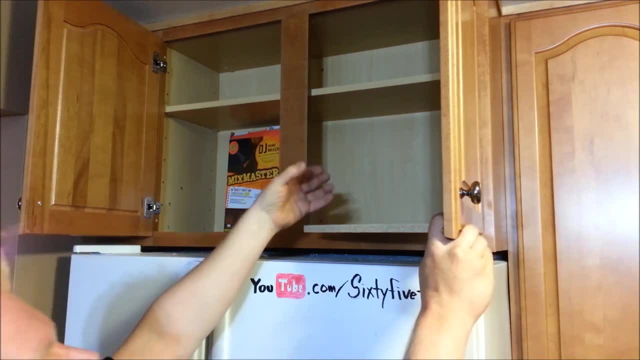 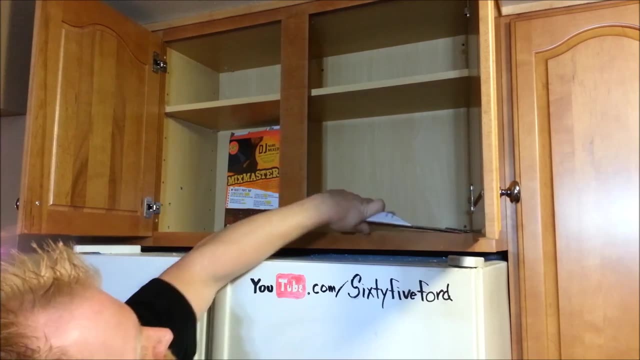 making it essentially a foot and a half, two feet closer, being right out here where I can reach it. So the first thing I did was make quite the elaborate cardboard template And I adjust sizes, take it to the door, Make sure it works. 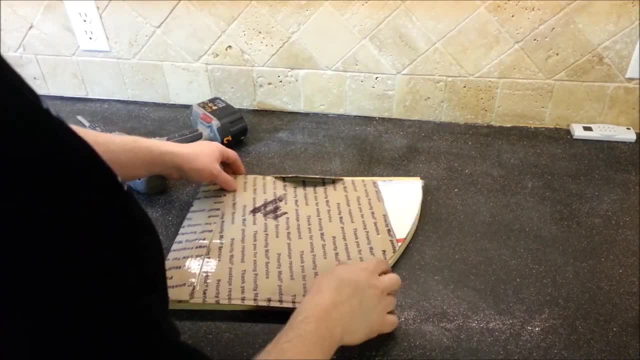 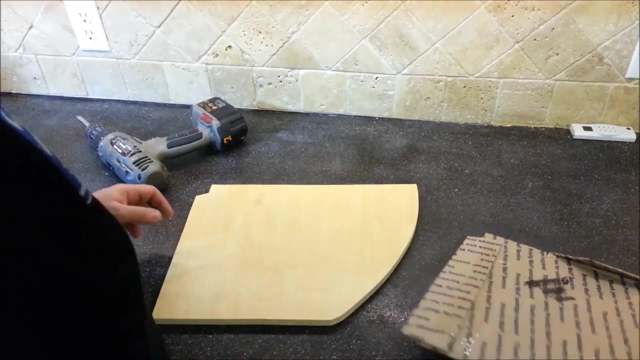 And came out with this And we took that and we just transferred it to a scrap piece of wood. This is just extra wood that I had Nothing fancy And also to keep stuff from falling off, I made a backer for it. 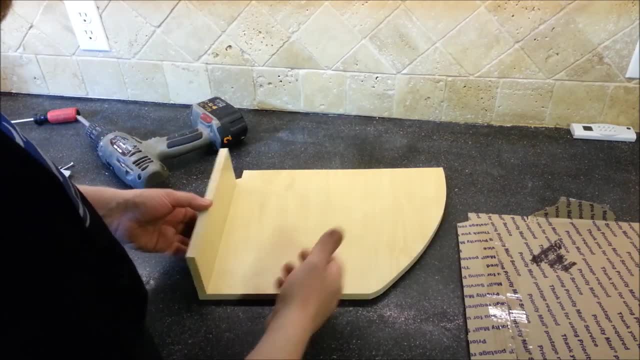 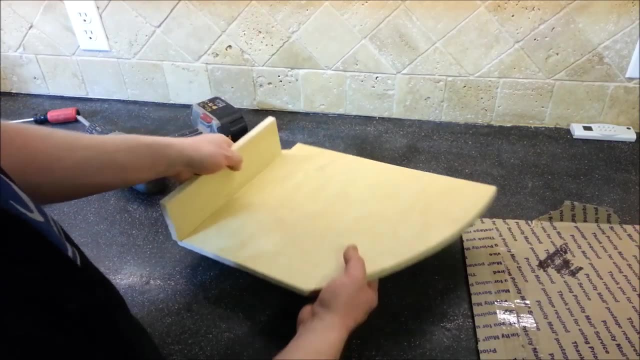 This will make some more sense, But just to keep stuff from falling off and on when you're closing, opening the door. But this I just screwed right there. I used pockets, but you can just screw it from underneath Whatever works. 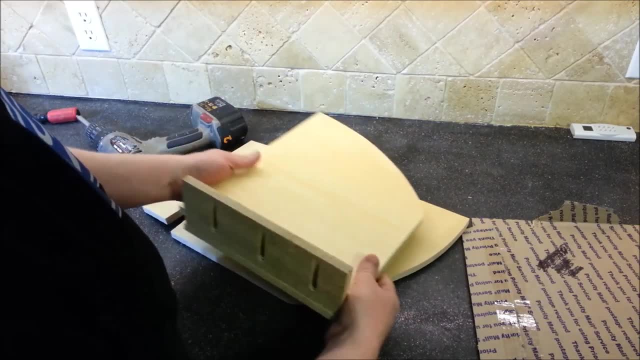 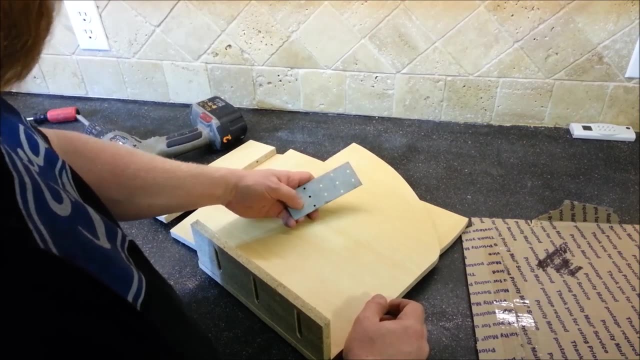 Not that important to even really have this, but it does help. And to mount this actually to the door, what I'm using is- this is just something I had lying around. They are like two by four ties, where you put two pieces of lumber together and you nail them in. 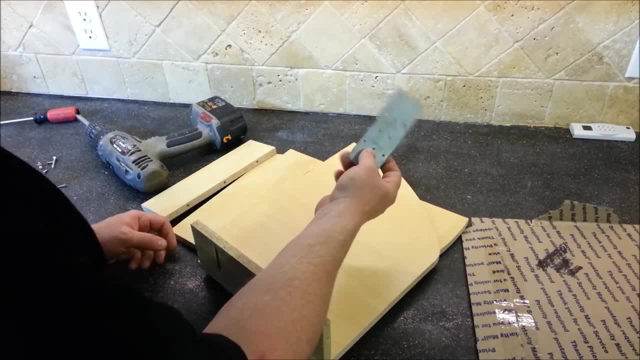 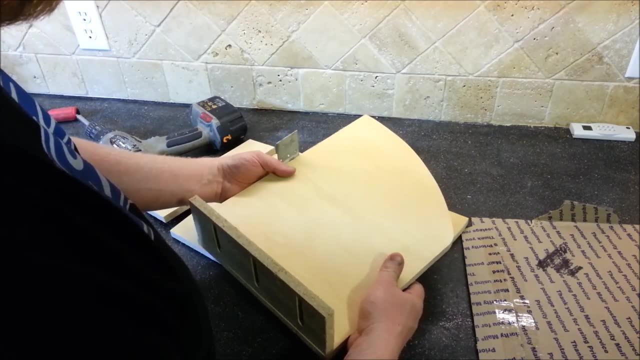 I think they're a quarter or something like that, 22 cents or something at the Home Depot those. I bent these at a 90 degree angle And what it'll do is it'll actually sit on the underside. Where's the front? Yeah, this is the front. 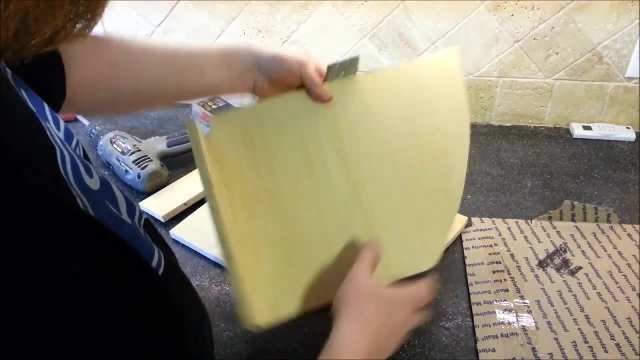 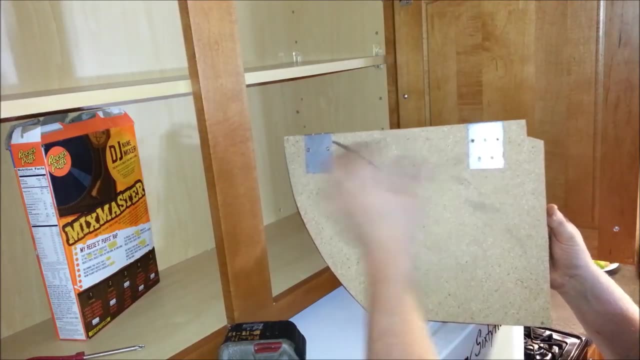 Sit on the underside. It'll screw to here and then it'll also screw to the door. So I've got the back panel mounted, I've got the little two brackets mounted. They're just screwed on. And now what I'll do is I'll just set this on here. 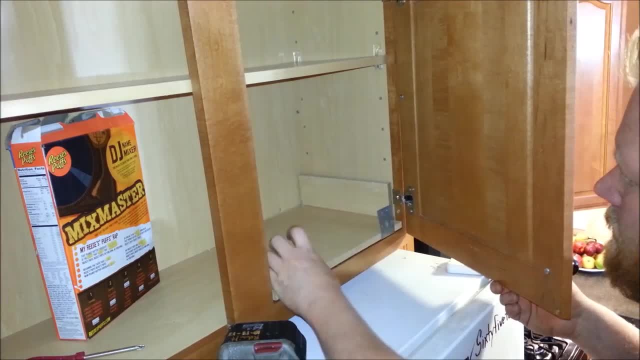 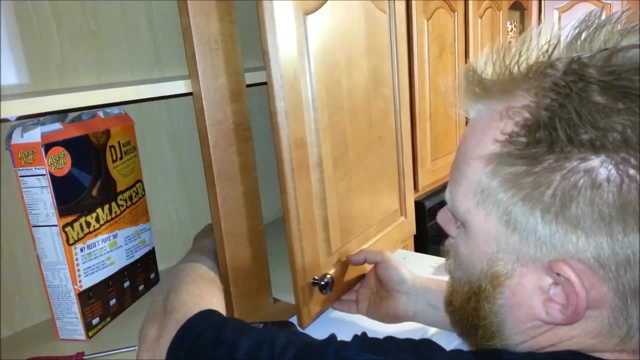 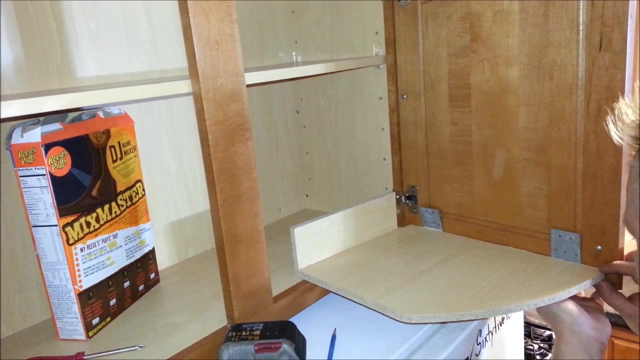 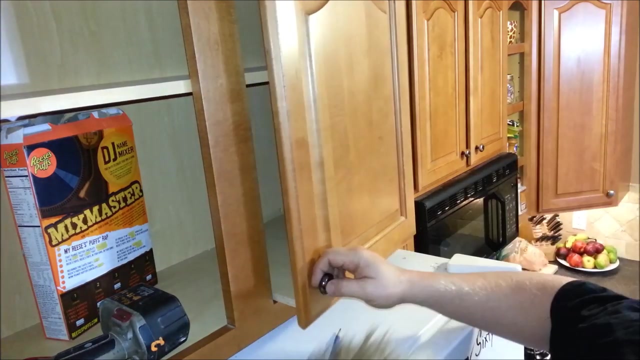 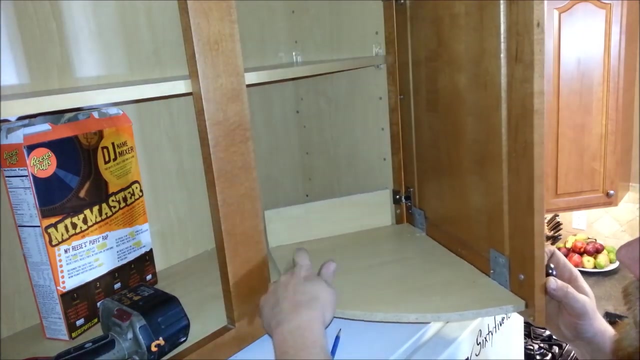 I'll close the door, Then I'll draw, Take my pencil and I'll mark where it needs to be And I'll just pull this out And we will screw it to the cabinet. There we go. Now the shelf actually is sitting here. 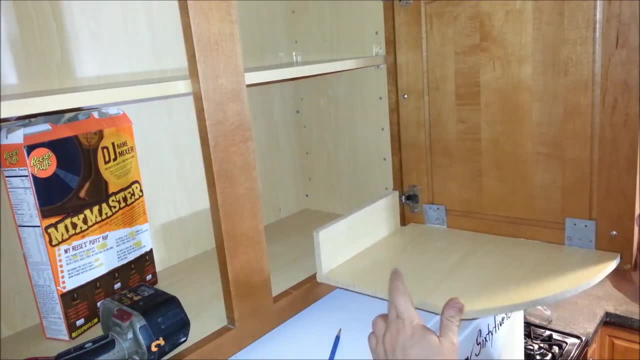 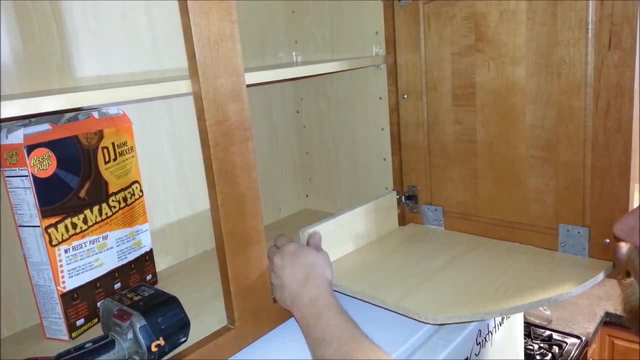 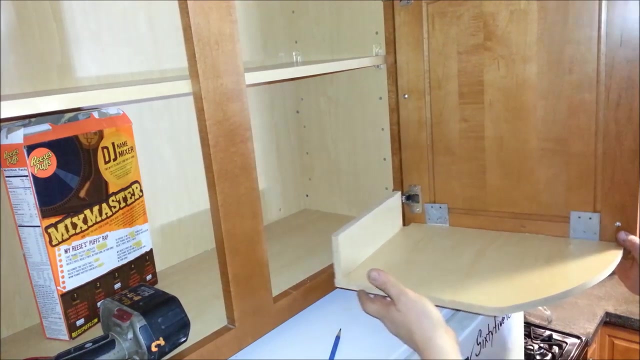 And you do have the problem with. as soon as it opens far enough, nothing is supporting it And you can let it just sit there. And if your doors only open about 90 degrees, this would be fine. But most doors these days with like Euro hinges and stuff, they will open up even further. 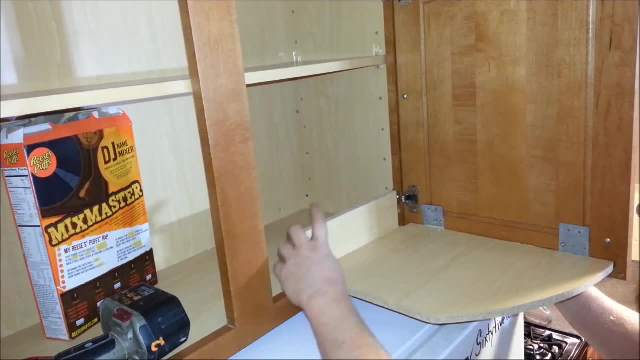 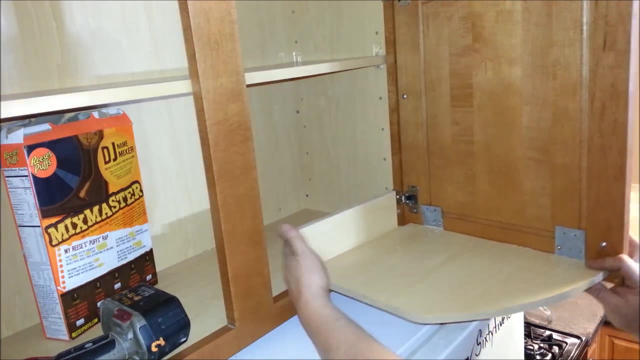 So I could. there's a couple options I could do. I could actually build a bigger back to it and actually screw it to the door. I could put a stop to limit the door from only opening. so far, What I'm going to do is: 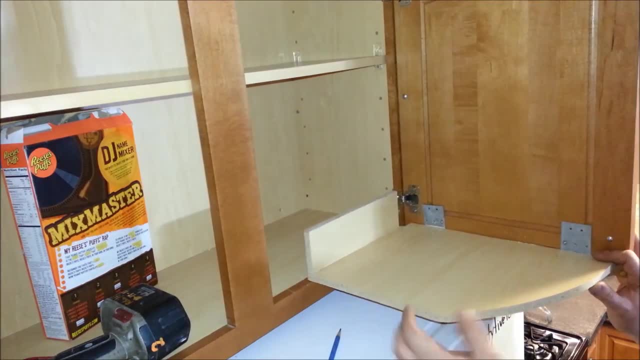 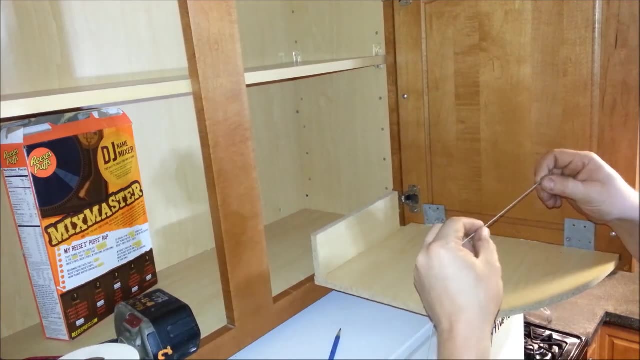 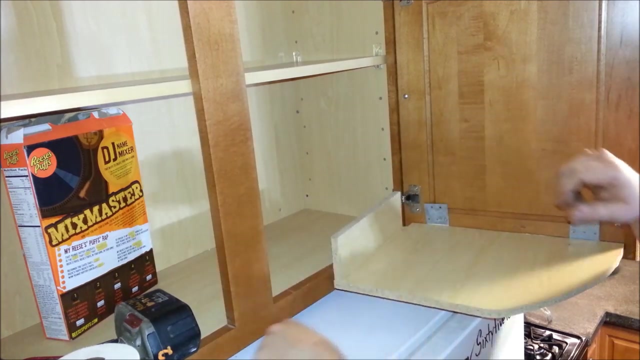 I like being able to open it this extra distance. I'm going to use heavy duty industrial string. This is actually- I believe this is extremely thin- paracord type stuff. Instead of the 550 pound, I believe it's like 90 pound or 100 pound. 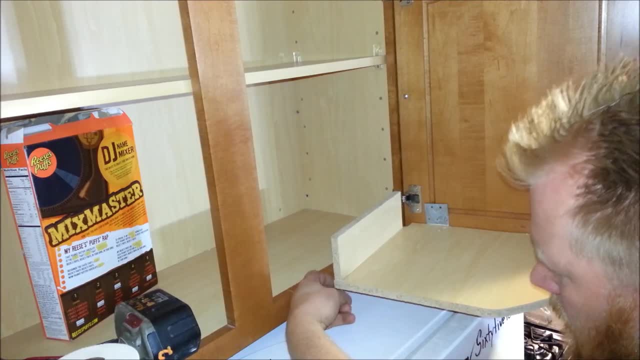 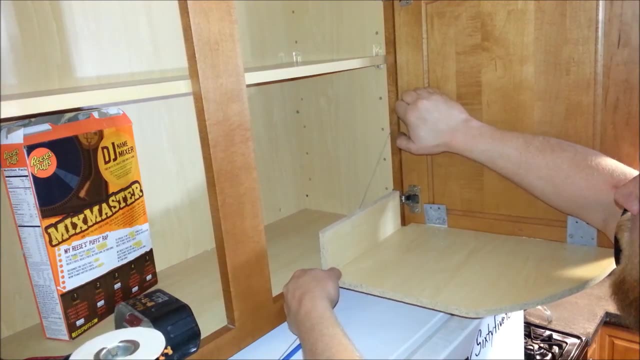 It's extremely strong. You can't break it by hand. What I'll do is I'll feed this up to make it so you can't really see, Because I'll actually just tie a knot And it'll support the weight of anything on there that you'll ever put on this drawer. 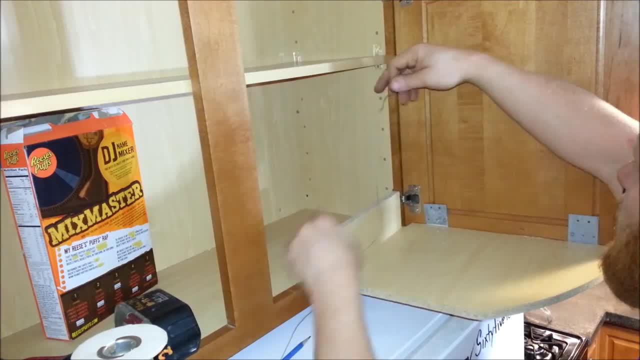 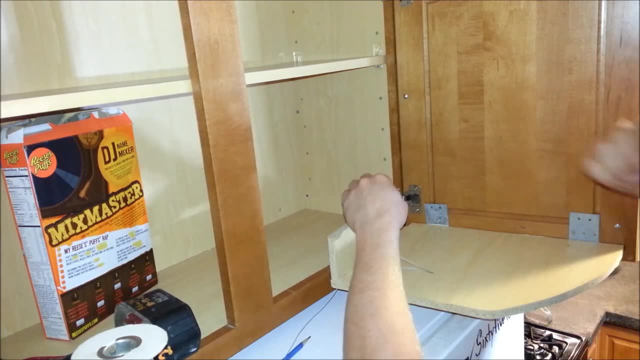 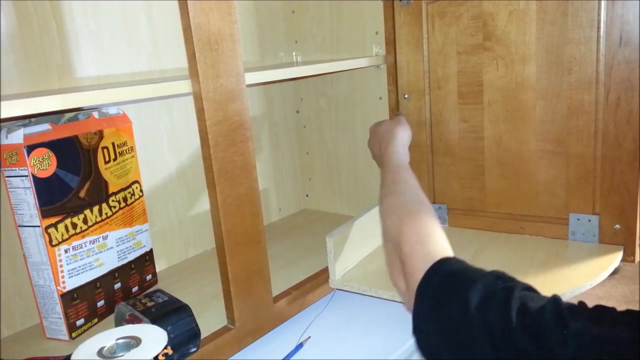 But it'll also act as a backstop. But I'll just tie, you know, a quick slip knot. What I did is I actually screwed a pan head screw up here, So I just tied a quick slip knot And I'll just feed that over there. 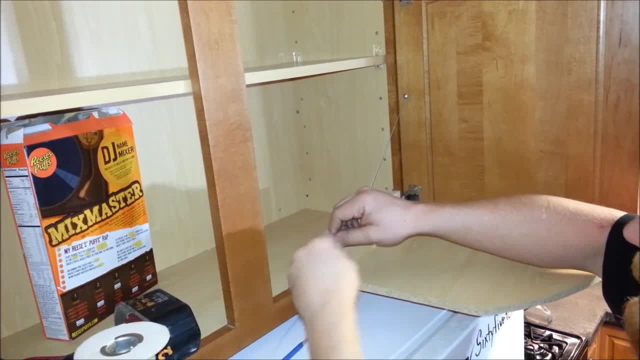 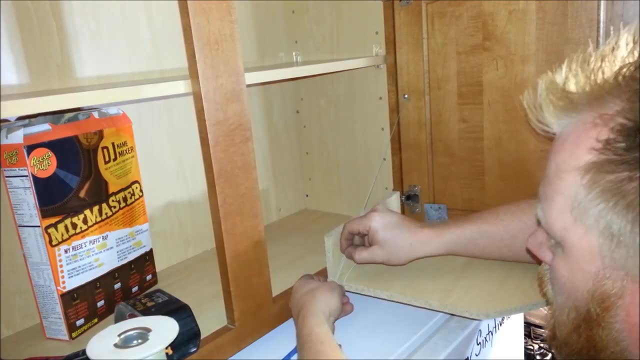 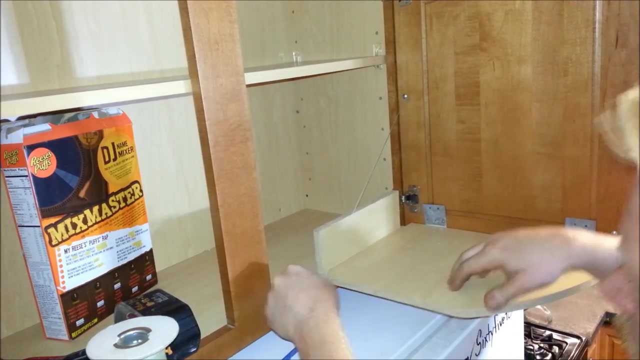 I'll bring this out, And I will. I'll actually loop it back through a couple times. Let's cut off the excess. I just drilled a roughly an eighth inch hole And you know, if it drags it doesn't really matter. 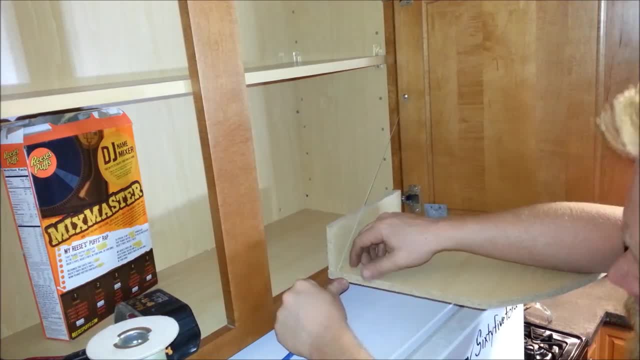 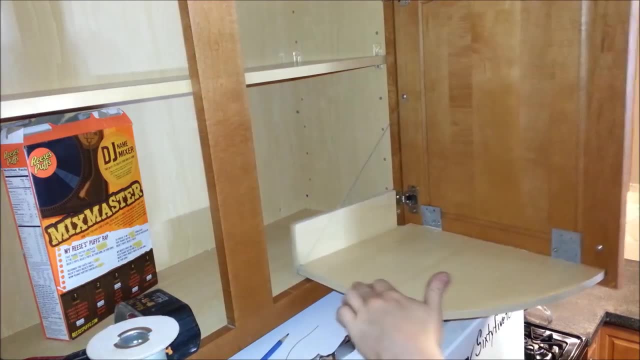 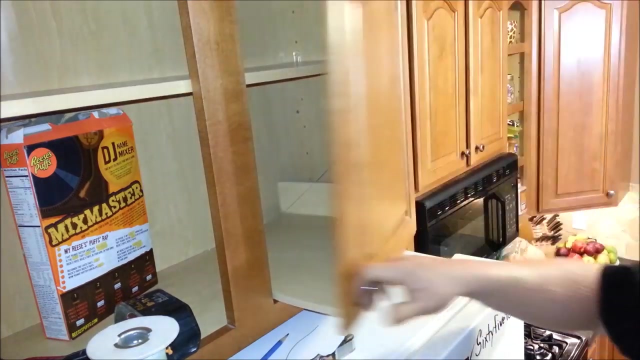 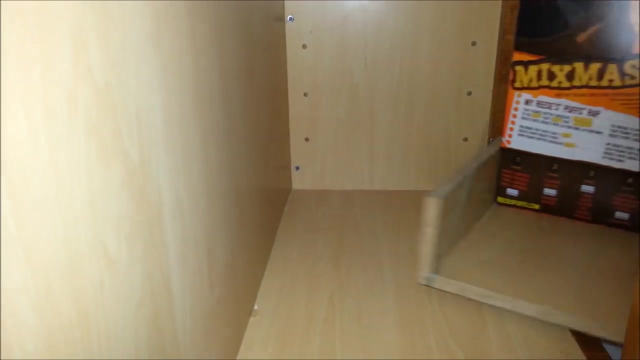 We'll pre-tension it, wrap it back through on itself a couple times, Get it to you know, There we go And I'll just hold the tension of whatever I put on there. But that's the idea And you can see when it closes in there. 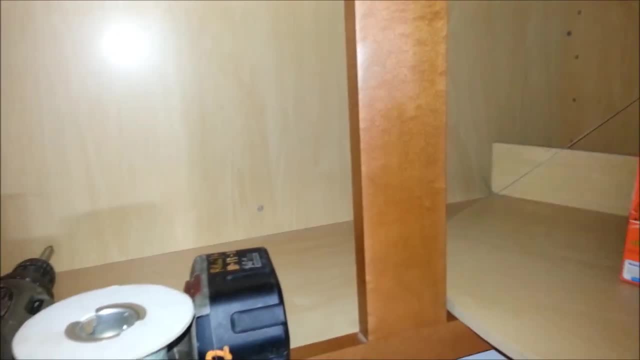 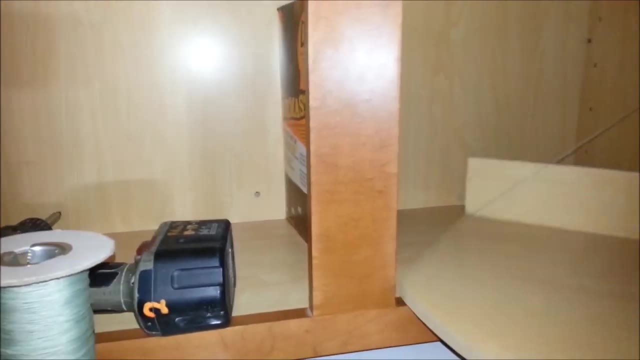 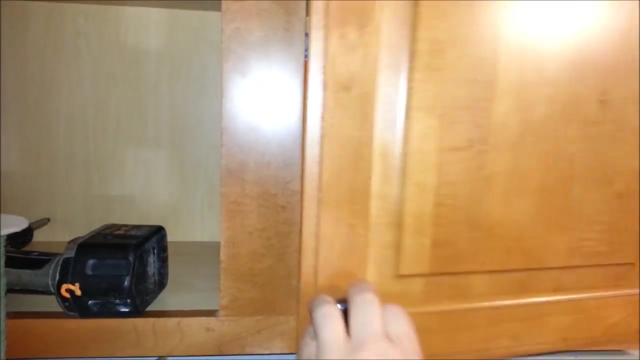 And that does leave a little extra space in the middle, But that you're not prevented from putting something in there. You know it doesn't rob it from you, It just doesn't slide out with you. But it stays in there just fine. 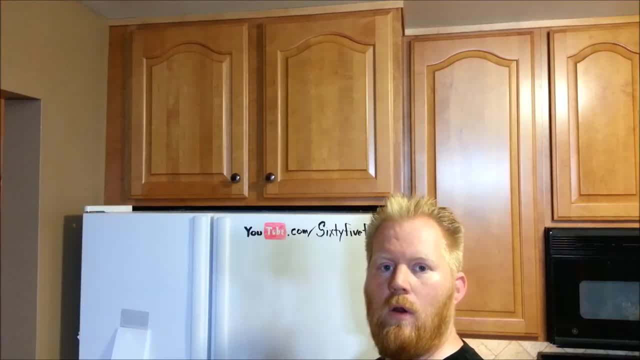 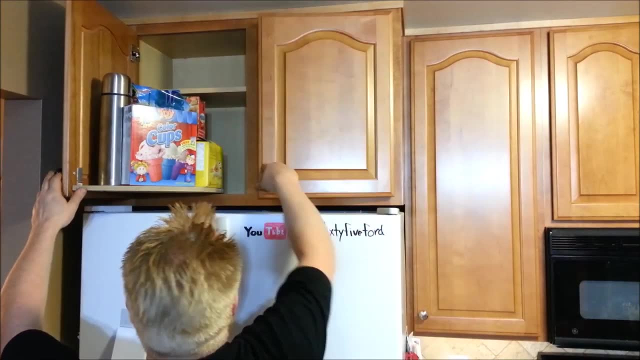 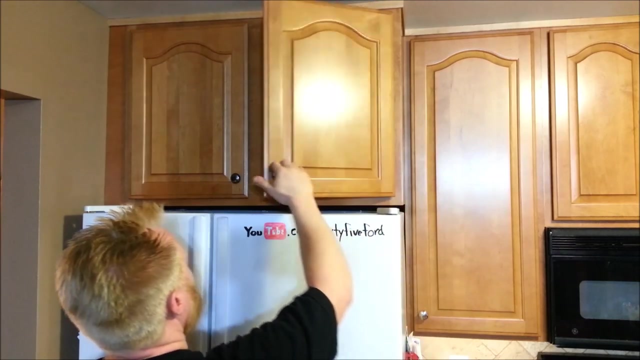 So now I'll do the other side. Well, there we go, guys. We take something that was virtually unreachable, unusable, And we turn it into something completely usable. There's no issues, You can't slam the door, But I mean you can shut them. 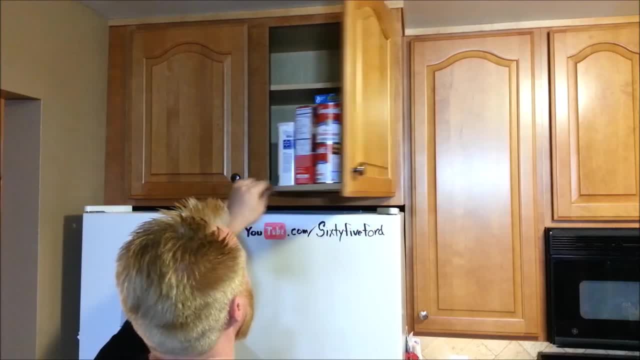 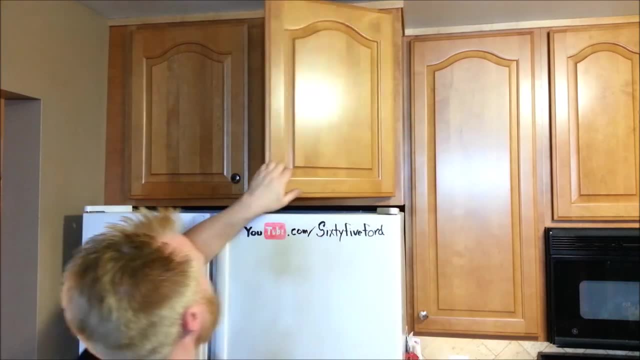 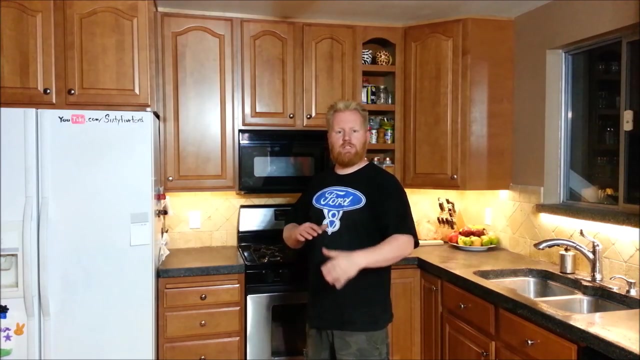 But you can't slam the door. But you can't slam it. You know all that stuff stays on there. Get me some crackers. There we go. Just a simple little woodworking project, No finishing, No major tools. Everything's hidden inside. 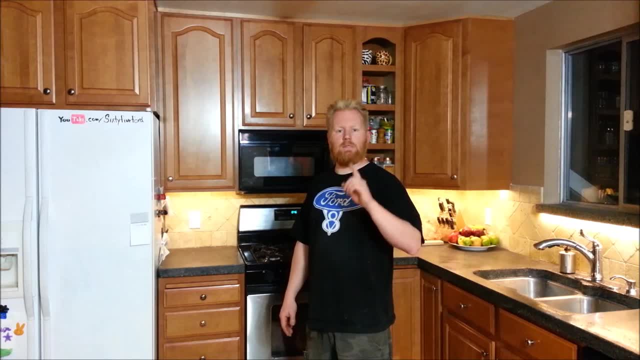 So it's more of a functional aspect More than a cosmetic, But it's awesome. Don't forget to share this on Facebook, Because your Aunt, Jodi, wants to see this And she wants you to come over and build her one. Don't forget to thumbs up love comment. 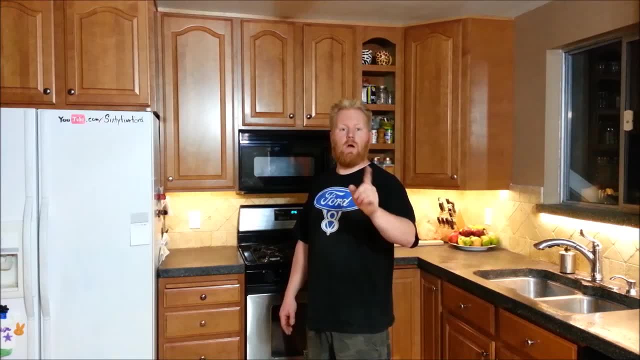 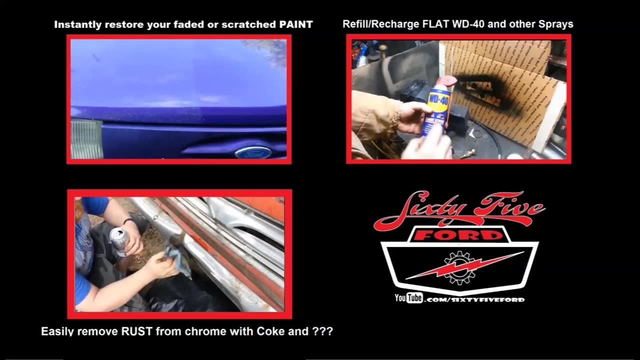 And check out my channel for a bunch of other awesome little builds Or some major builds that I've done in the past. Thanks guys, See you soon. Bye. .